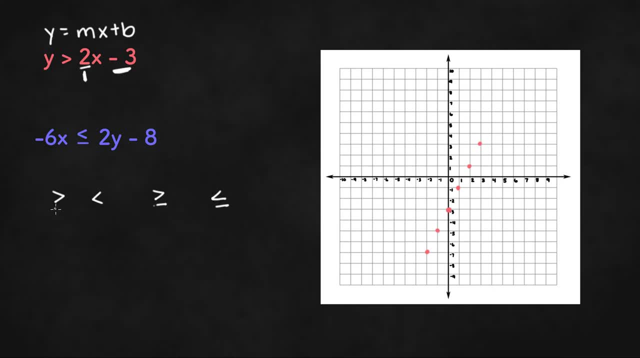 And less than and less than or equal to. So greater than and less than will be a dashed line That shows that it's not equal to 2x minus 3.. It's just greater than And greater than or equal to, and less than or equal to will be solid lines. 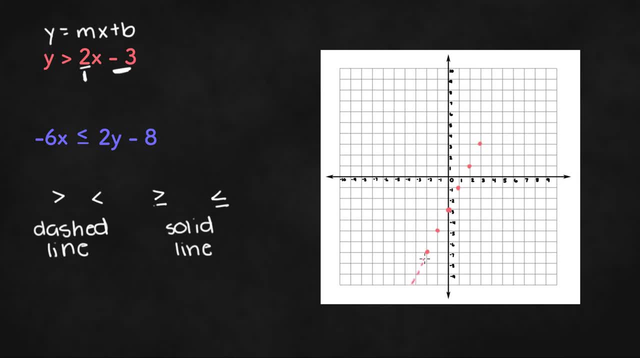 So we can kind of graph a dotted line like this Or a dashed line. Now, since the y is greater than this value, we have to shade above the line. This shows that everything above the line is greater than, And this dotted or dashed line shows that it's not equal to. 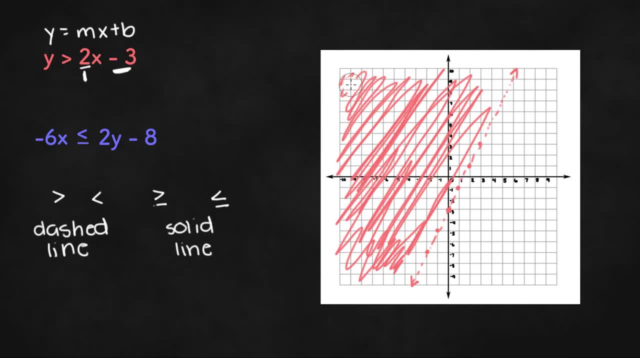 It's only greater than Now. the next equation is negative: 6 is less than or equal to 2y minus 8.. So we can get that in slope-intercept form by adding the 8 to both sides. That leaves us with negative: 6x plus 8 is less than or equal to 2y. 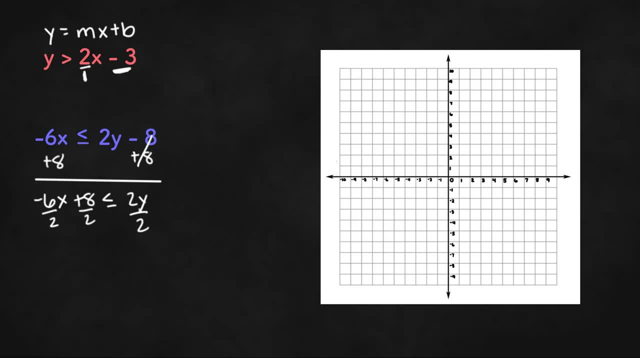 And we can divide all the terms by 2. And we have negative. 3x plus 4 is less than or equal to y. Now we can also flip this equation so that it looks more like y equals mx plus b. We don't have to change anything. 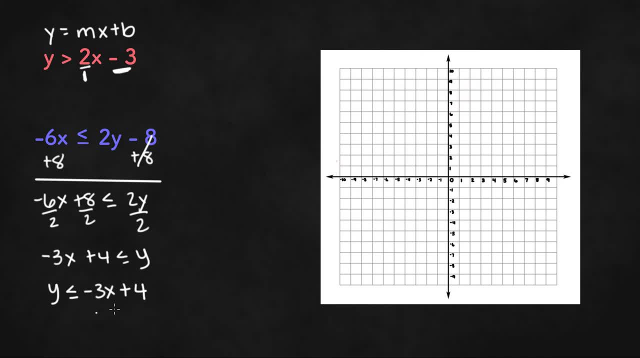 Now we can plot the point 4 for the y-intercept And then negative 3 over 1. So that would be down 3 and right 1.. Down 3 and right 1. Or up 3 and left 1..